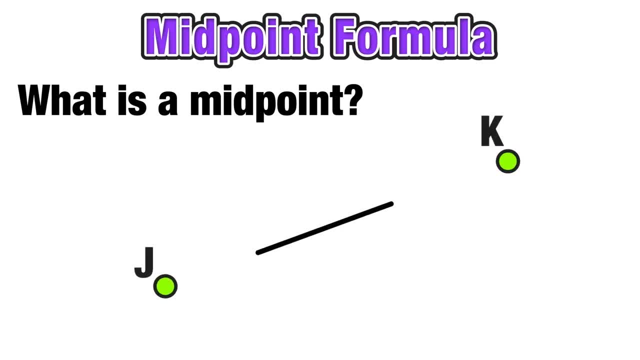 Now we can extend this thinking to finding the midpoint of a line segment that connects two points, by finding the point that is directly in the middle of the line segment, such that it cuts it into two congruent halves. In this case you have line segment JK. point M is 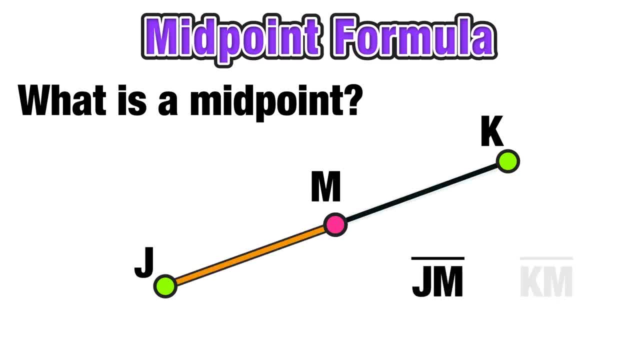 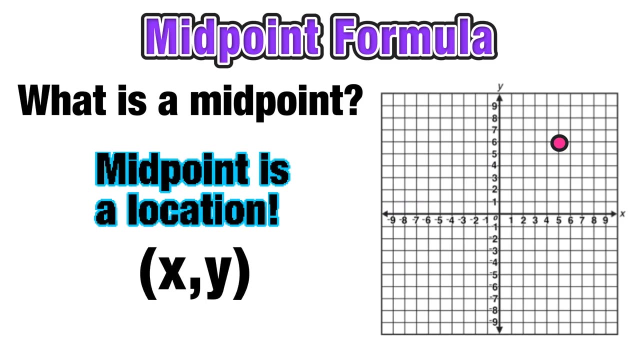 directly in the middle, so that JM is one half KM is the other half, and they are both congruent. Now we are going to be concerned with finding midpoints on the coordinate plane, So we want to think of a midpoint as a location with XY coordinates. 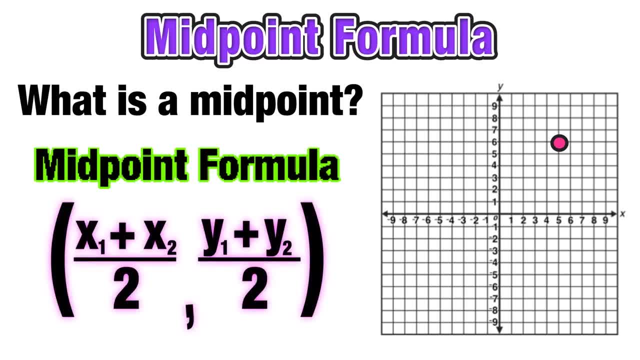 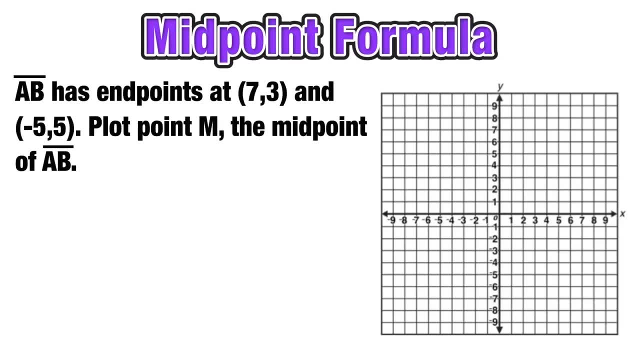 And our tool in this lesson for finding the midpoint is going to be the midpoint formula, So let's go ahead and learn how to use it. Our first example wants us to find the midpoint of line segment AB, and it's giving us the coordinates of both endpoints. 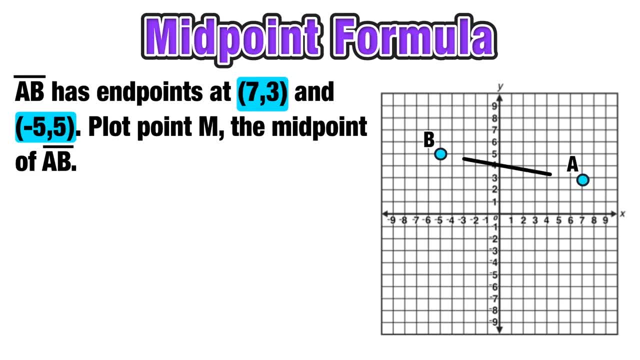 So let's start by plotting those endpoints, A at and B at, and then constructing line segment AB. So we want to find the midpoint of this line segment. again, we want to find the XY coordinate that is directly in the middle of this line segment, such that it cuts it into two congruent 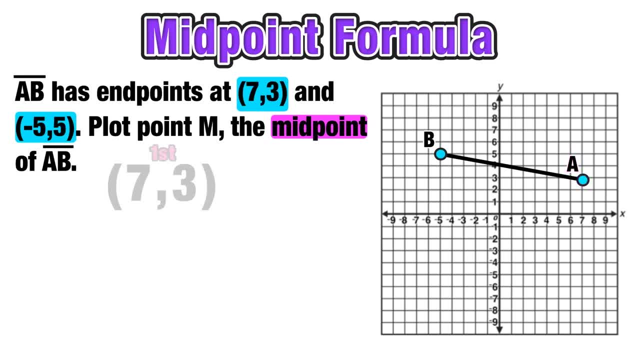 halves. Let's go ahead and write down the coordinates of A, our first point at, and B, our second point at. Now we are prepping ourselves to substitute the right values into the midpoint formula. Now endpoints A and B are just x and y. 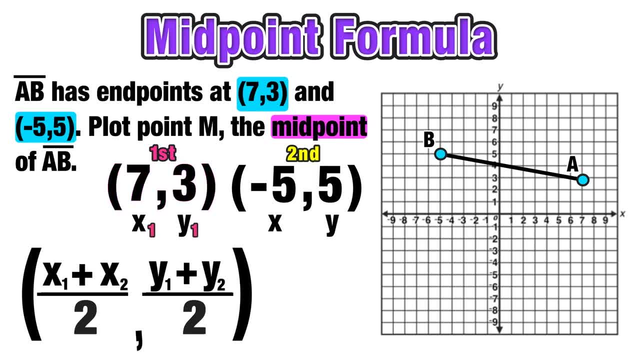 Since the first point was the first point, that's going to be the x1, y1. And since negative 5, 5 was the second point, that's going to be our x2, y2.. Now on the left side, x1 plus x2 is just going to be 7 plus negative 5.. 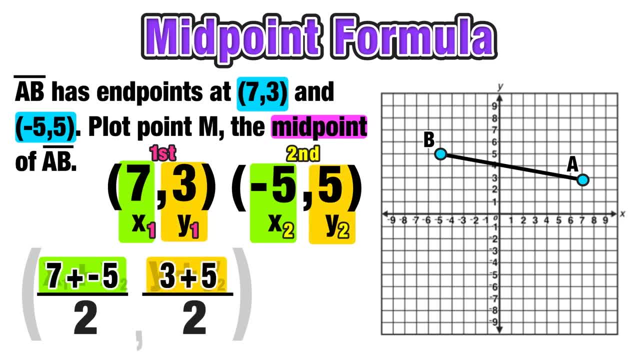 On the right side, y1 plus y2 is just 3 plus 5.. We can continue to evaluate: 7 plus negative. 5 equals positive 2,. over on the right side, 3 plus 5: just equals negative. 2. Just equals 8.. 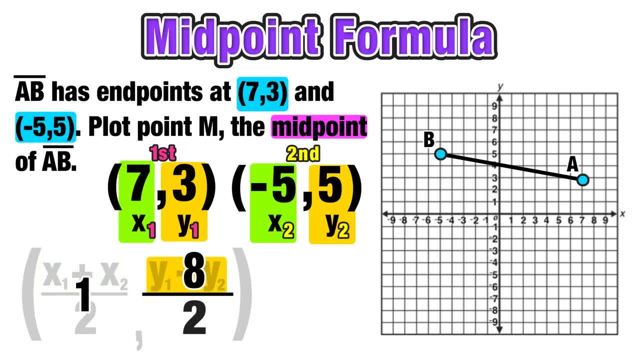 And finally, 2 divided by 2 or 2 over 2 is just 1.. And over on the right, 8 divided by 2 or 8 over 2 is equal to 4.. So using those two endpoints in the midpoint formula, we have found the coordinates of: 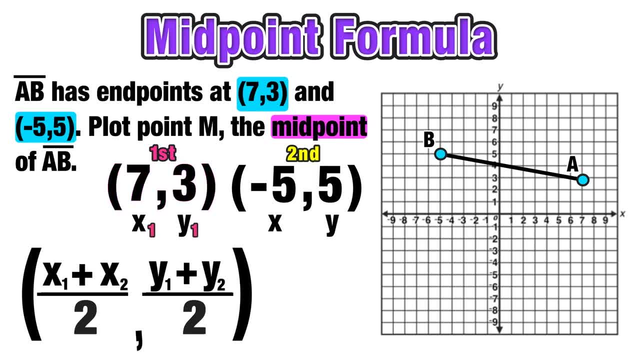 Since the first point was the first point, that's going to be the x1, y1. And since negative 5, 5 was the second point, that's going to be our x2, y2.. Now on the left side, x1 plus x2 is just going to be 7 plus negative 5.. 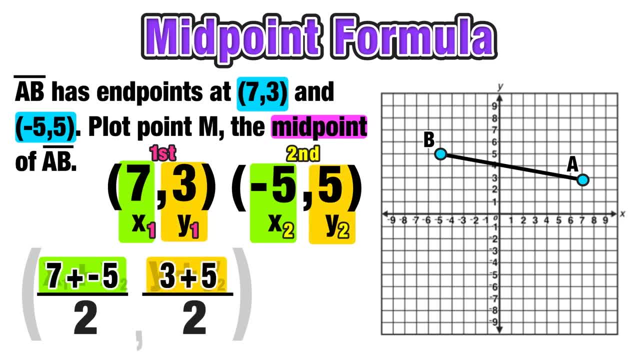 On the right side, y1 plus y2 is just 3 plus 5.. We can continue to evaluate: 7 plus negative. 5 equals positive 2,. over on the right side, 3 plus 5: just equals negative. 2. Just equals 8.. 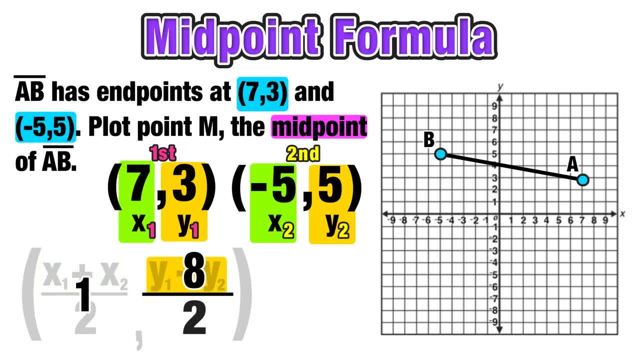 And finally, 2 divided by 2 or 2 over 2 is just 1.. And over on the right, 8 divided by 2 or 8 over 2 is equal to 4.. So using those two endpoints in the midpoint formula, we have found the coordinates of: 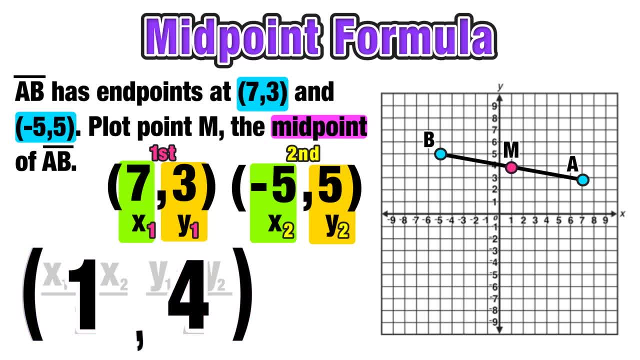 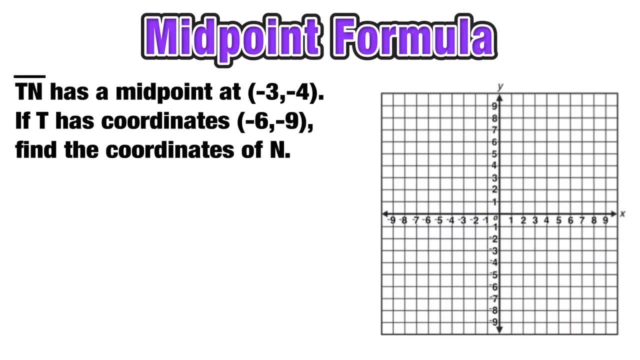 the midpoint of line segment A B at Now. our final example is slightly more advanced than the previous one. It's a little bit more complex than the previous one. It's a little bit more complex than the previous one. It's a little bit more complex than the previous one. 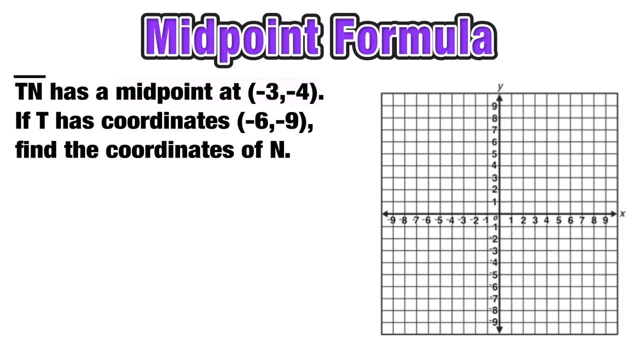 So let's go ahead and take the example that we just completed. This question is not asking us to find the midpoint. it's giving us the midpoint of line segment TN at. It's also giving us the coordinates of one of the endpoints- this case T with coordinates. 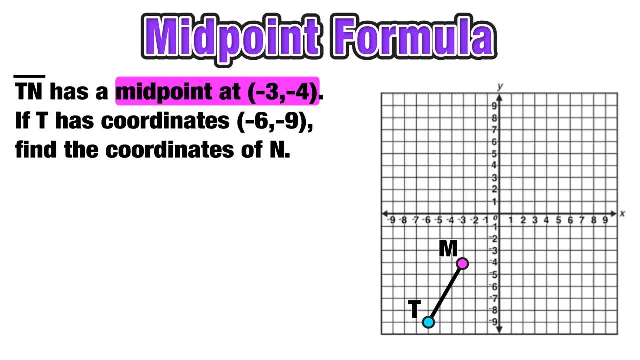 What we want to find is the coordinates of the other endpoint N. So let's visualize what's going on here. We know where the center of the line segment is. we know one of the endpoints. we want to find the other endpoint n. So we know that endpoint. 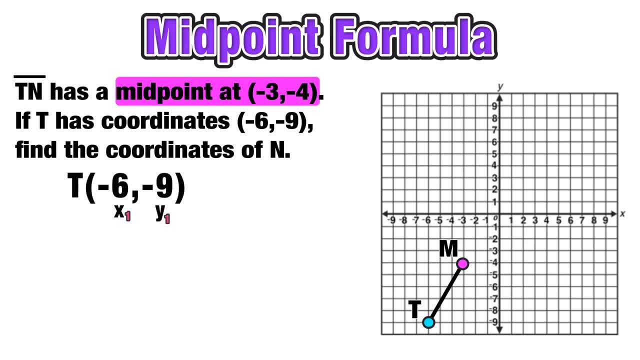 t has coordinates at negative 6, negative 9, that's our x1, y1. And our other endpoint, n, has unknown coordinates, but that's still going to be our x2, y2.. Now we're still going to use the midpoint formula, but we know that it's going to equal the midpoint which we 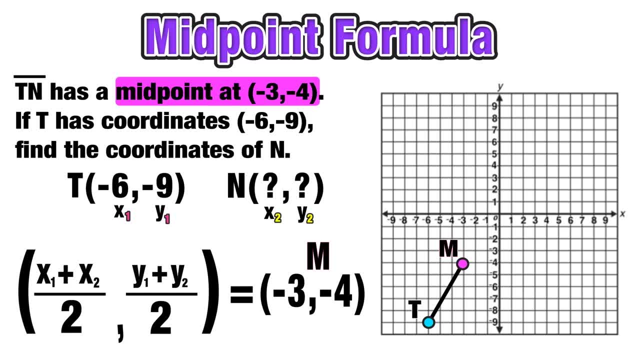 already have, which is negative 3, negative 4.. So we'll start with the x coordinate of the midpoint at negative 3.. So we know that negative 6 plus some unknown number, divided by 2, would have to equal negative 3.. Solving this algebraically shows us that the unknown 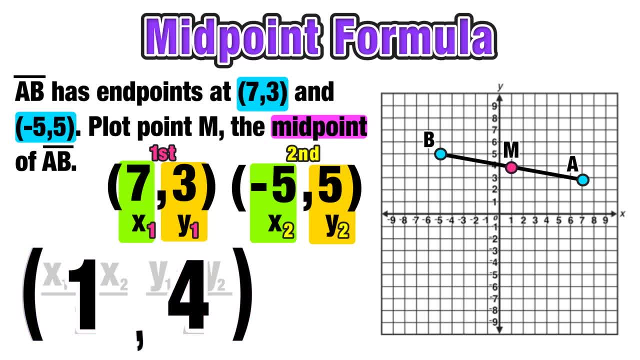 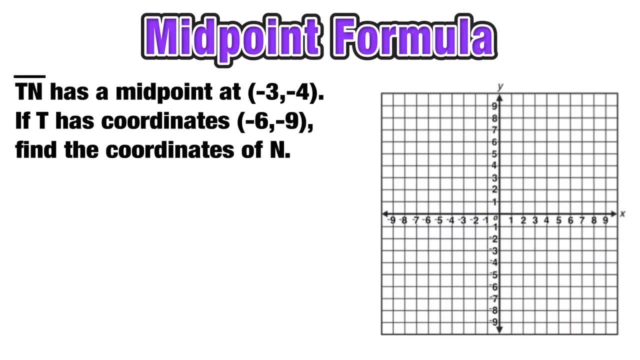 the midpoint of line segment A B at Now. our final example is slightly more advanced than the previous one. It's a little bit more complex than the previous one. It's a little bit more complex than the previous one. It's a little bit more complex than the previous one. 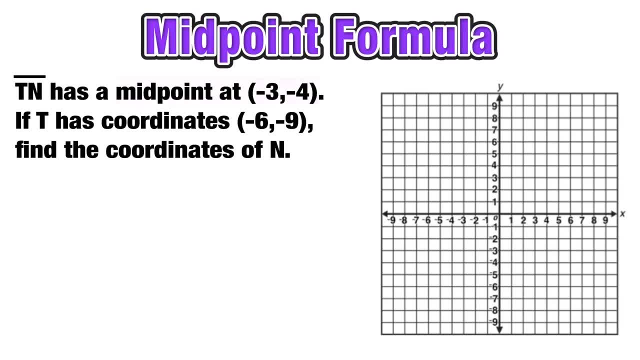 This is the first example that we just completed. This question is not asking us to find the midpoint. it's giving us the midpoint of line segment TN at. It's also giving us the coordinates of one of the endpoints. this case T with coordinates. 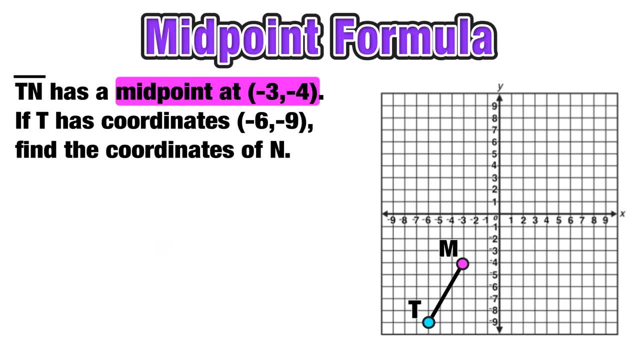 What we want to find is the coordinates of the other endpoint N. So let's visualize what's going on here. We know where the center of the line segment is And we know one of the endpoints- endpoints we want to find the other endpoint n. So we know that endpoint t has coordinates. 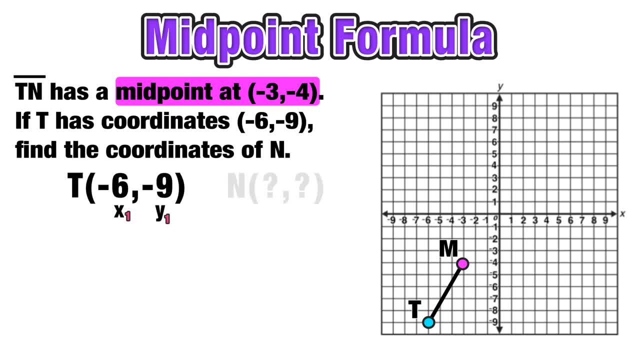 at. that's our and our other endpoint n has unknown coordinates, but that's still going to be our. Now we're still going to use the midpoint formula, but we know that it's going to equal the midpoint which we already have, which is: 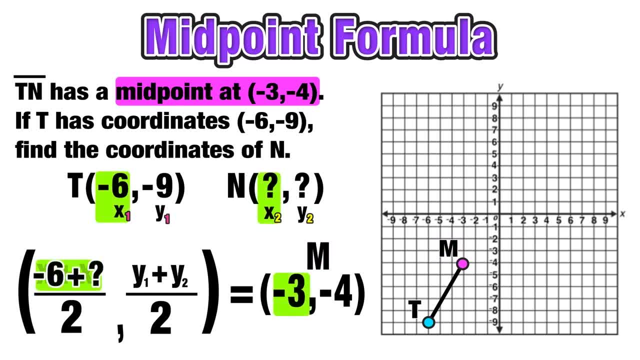 So we'll start with the x-coordinate of the midpoint at. so we know that negative 6 plus some unknown number, divided by 2 would have to equal negative 3.. Solving this algebraically shows us that the unknown number will be 0, since negative 6 plus 0 is just negative 6,. 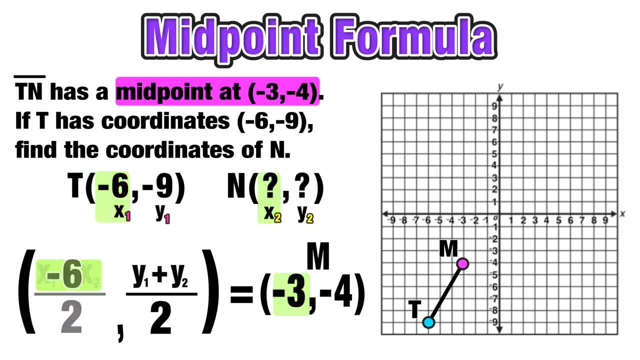 and negative. 6 divided by 2 does equal negative 3.. So what we just did was confirm the x-coordinate in the midpoint, the, And we know that the value of the x-coordinate in endpoint n is 0.. Next we want to find the value of y2 in endpoint n. Now we know that the y value in the midpoint 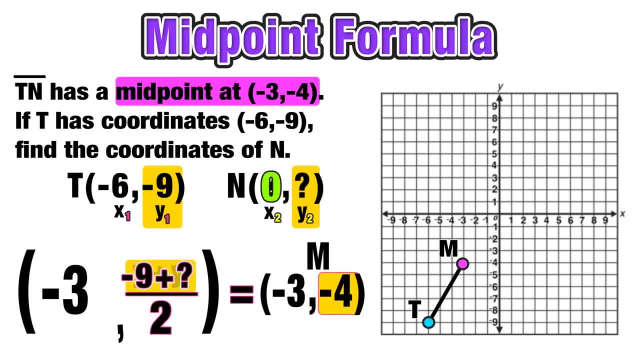 is negative 4, so we just want to find negative 9 plus what unknown value. divided by 2 is going to equal negative 4.. When we solve this algebraically, we should get positive 1 for that unknown value, since negative 9 plus 1 is equal to negative 8..